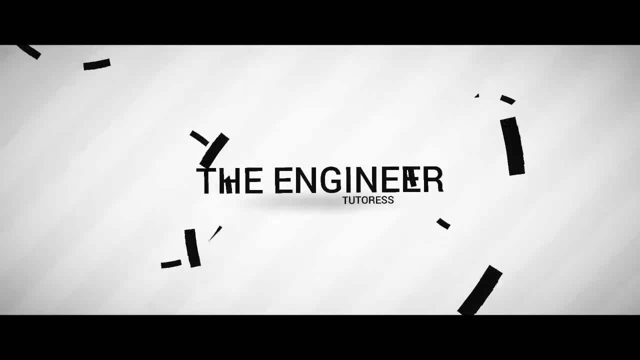 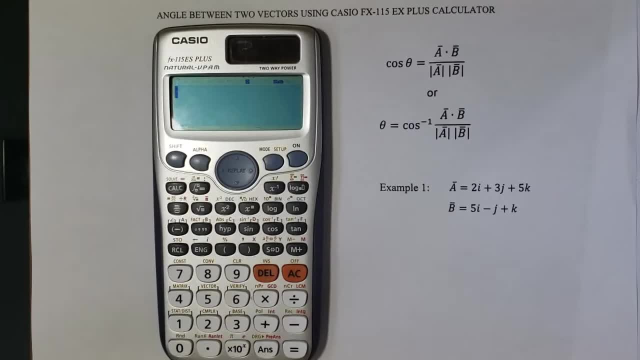 Welcome everyone. In this video we will work on a problem: to find the angle between two vectors using Casio FX115ES Plus calculator. Also, I will show you a shortcut of how to find the magnitude of the vectors Instead of doing it manually and moving between modes. we will do. 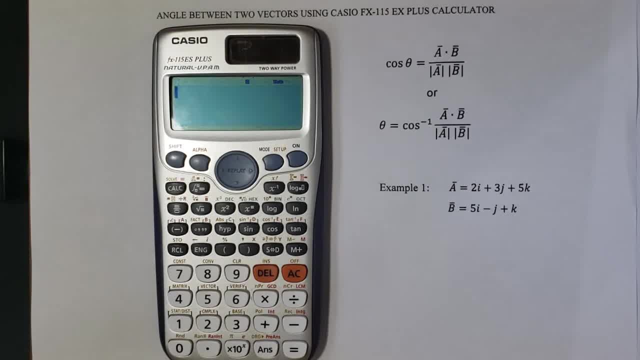 everything in a vector mode. Before doing the example. if you want to find the angle between two vectors, we use this equation. here We can see, on the left side of the equation we have cosine of the angle and on the right side we have a fraction. We will take the dot product. 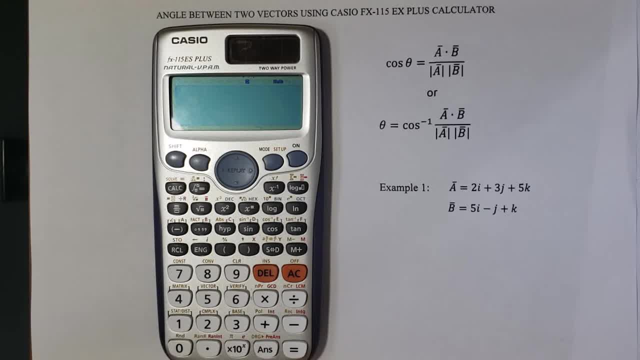 between the two vectors in the numerator and we will take the product of the magnitudes of both vectors. So let's say we were given these two vectors here, vector A and vector B. We need to insert these values in our calculator. I will go to mode here and I will press 8 for 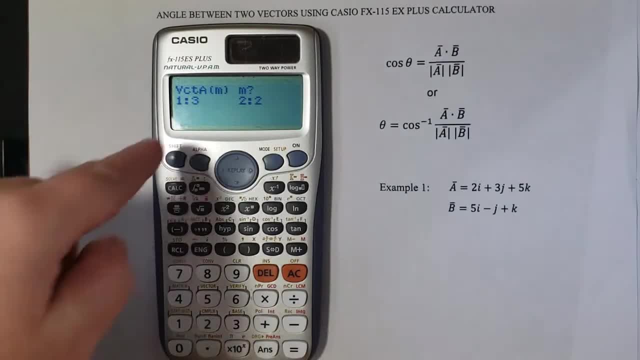 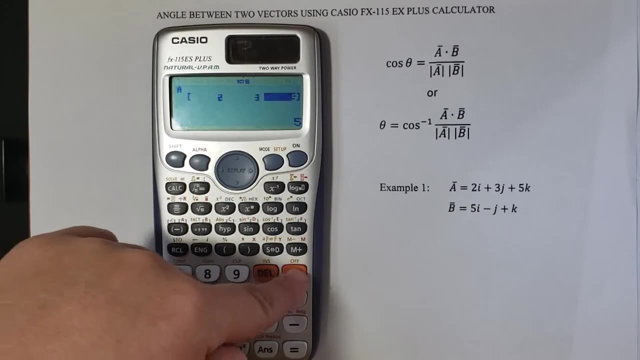 vector and 1 for vector A, and then 1 again for the three directions of the vector. So 2 equal, 3 equal, 5 equal. I will press the all clear button here in order for the calculator to save these values. Now mode again: 8. and now 2 for vector B and then 1 for the three directions. We have 5. 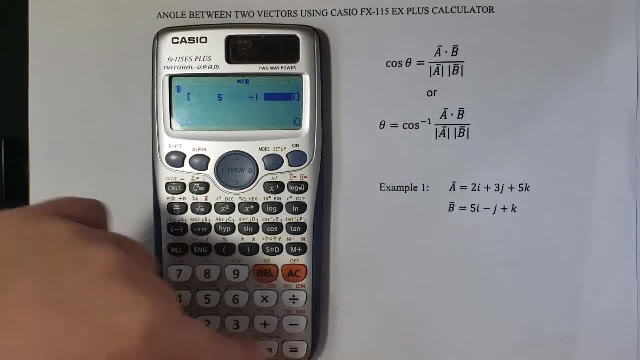 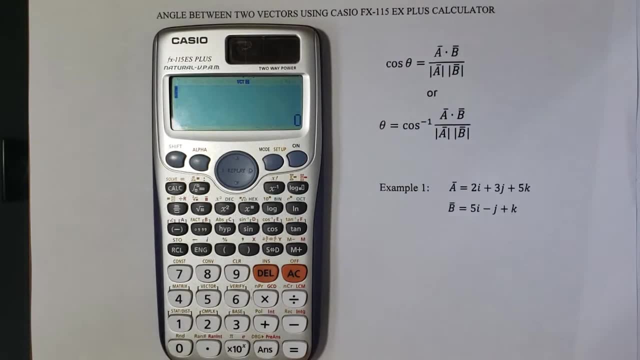 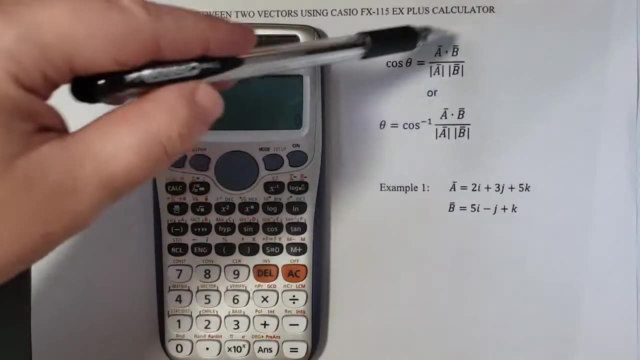 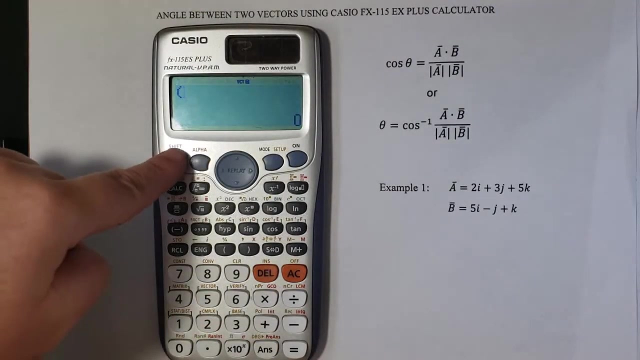 equal minus 1. equal 1, equal All. clear button to save. Now I will open a parenthesis and I will in the calculator. I will insert everything that's here on the right side of the equation. So we have a dot product of the two vectors. I'll press shift. 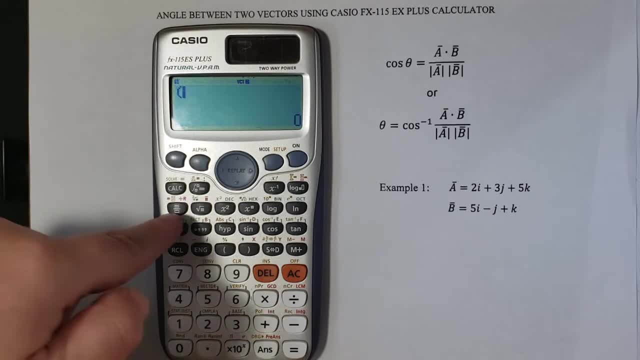 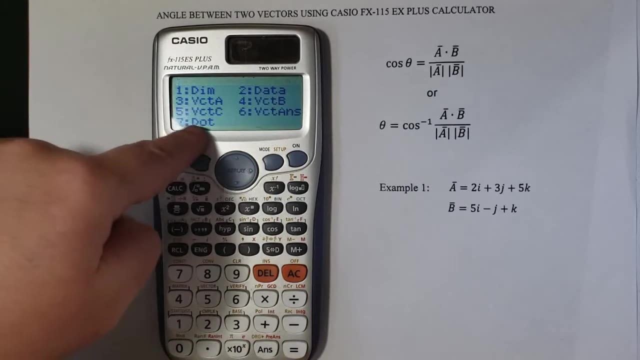 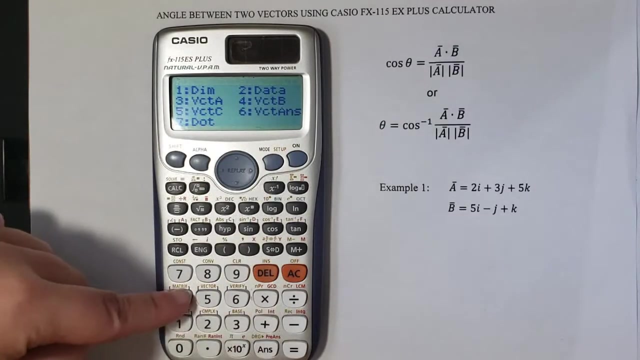 key. This shift key here is used to access each of the yellow options above each key. So shift, and you see 7 is for dot, So 7.. Shift again. Vector 4 for vector B: Close. Next in our equation is: 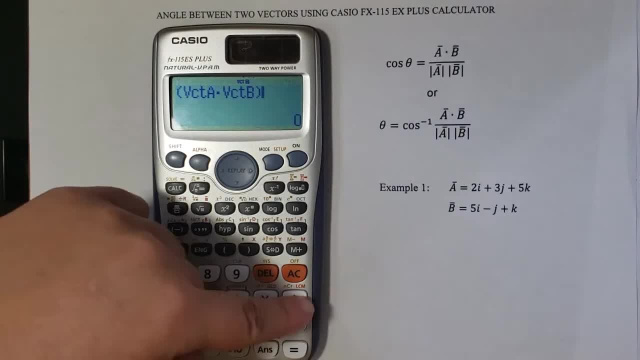 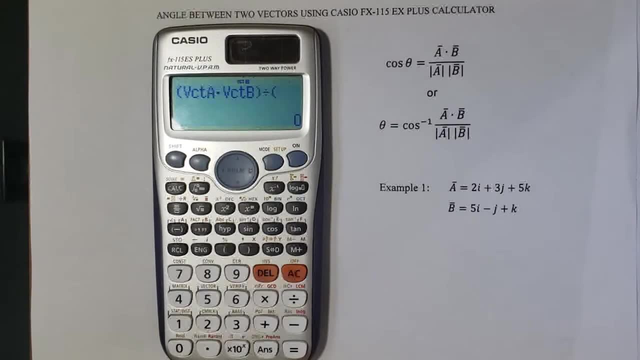 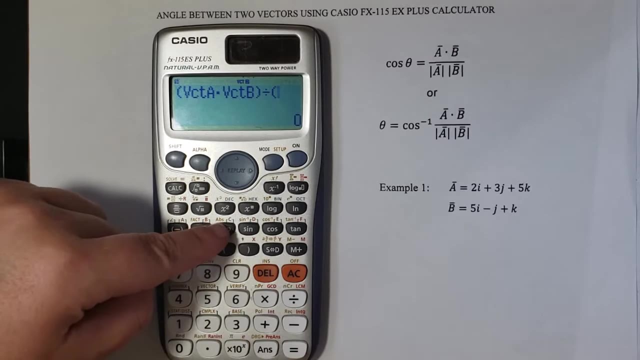 the denominator. So I will divide it by the magnitudes of both vectors and their product. And how can I find the magnitude of a vector? I'll press shift and you see this absolute key here. That is how you can find the magnitude of a vector. So absolute Shift again. Vector. 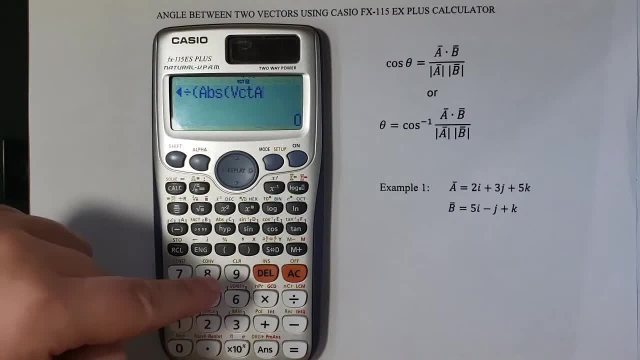 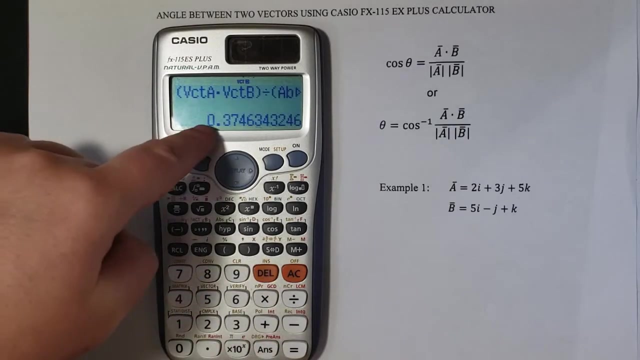 3 for vector A, Close, And then a product, So times the absolute or the magnitude of vector B, Shift again Vector. and then 4 for vector B, Close and close again. I will press equal. This value is a cosine of theta. In order to find the angle theta. 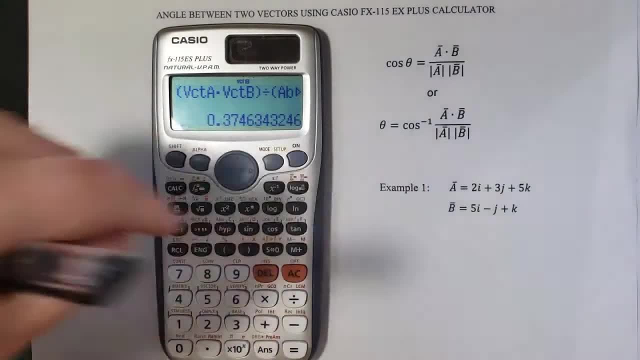 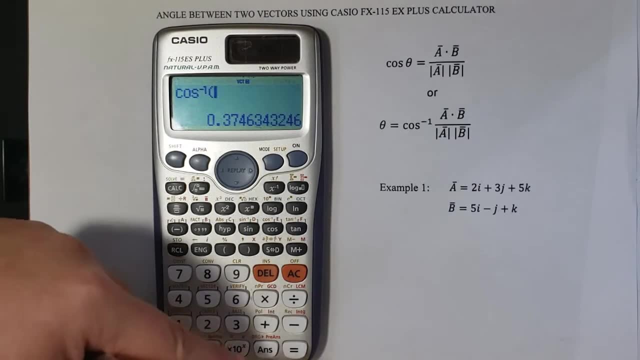 we simply need the inverse of the cosine, Then shift. I'll press this button, cosine here, And then now I'll press this answer memory key here, This button, this memory helps the result of a calculation. after the equals key, So close the parentheses and then equal 67.99.. That is how much is the angle between. these two vectors. Thanks for watching.